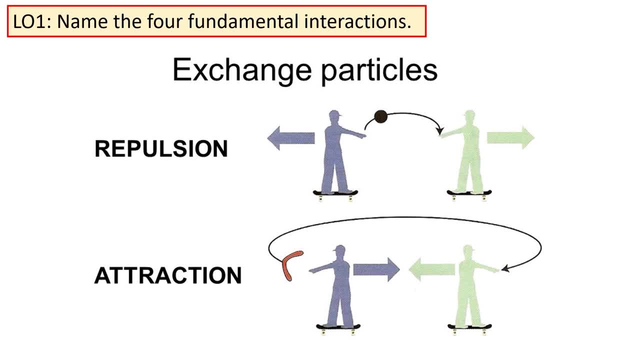 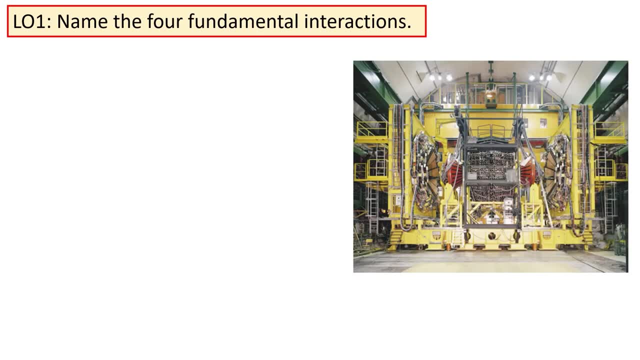 particle that is passed between two other particles which then experience the force. The other exchange particle we should be aware of is the W boson. The W boson is responsible for mediating the weak nuclear force. The W boson has a non-zero mass. It also has a very, very short 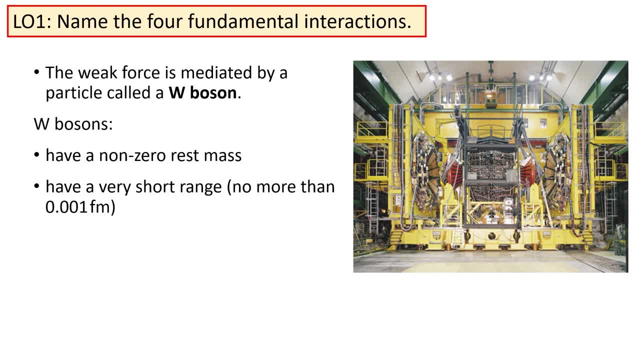 range about 0.001 femtometers. It can also be positively or negatively affected by the energy of a particle. It can also be positively or negatively charged, which will be very important when we consider conservation laws later in the topic. Similarly, you should also be aware that the 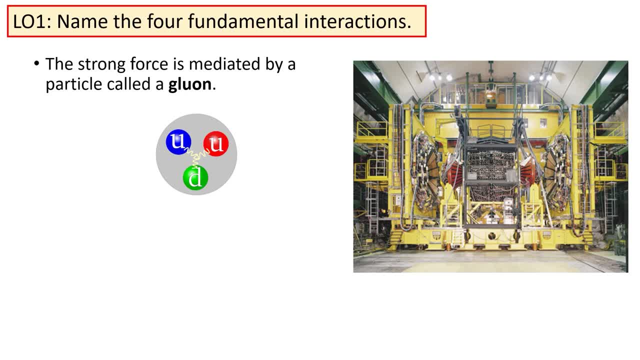 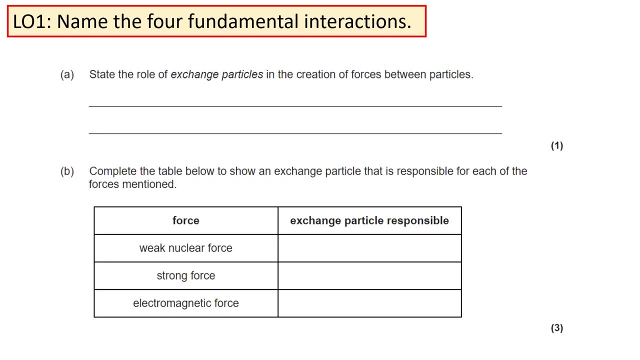 strong nuclear force is mediated by a particle called a gluon. For historical reasons, you may sometimes see this written as a pion. We also have a hypothetical particle which mediates gravity, called the graviton. This is yet to be detected directly. Here's a chance for you to have a go at a question. 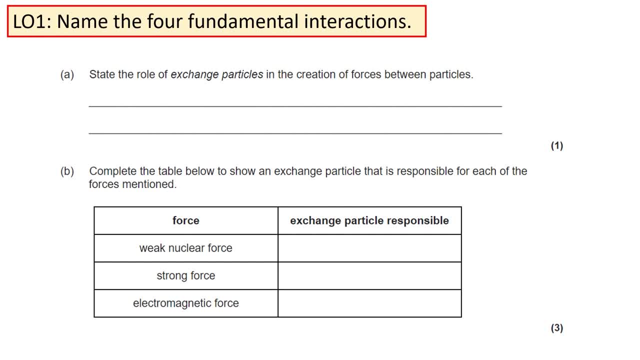 Here's a chance for you to have a go at a question. Pause the video and write an answer for each of these questions. I'll give you a second to do that and then I'll give you the answers. And here are the answers to that last question. 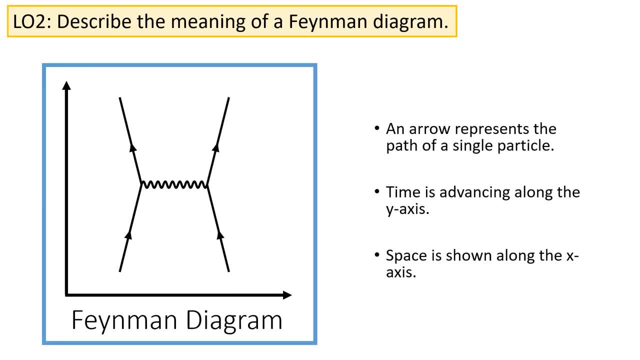 Next up we have Feynman diagrams. Feynman diagrams are a convenient way to represent the interactions between particles. On a Feynman diagram, an arrow represents the path of a single particle. On the y-axis we have time advancing and on the x-axis we have space. Generally speaking, however, 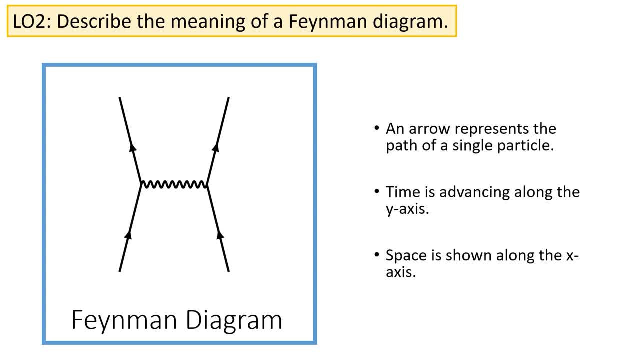 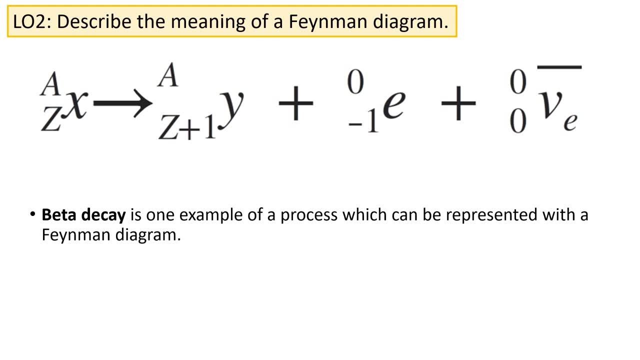 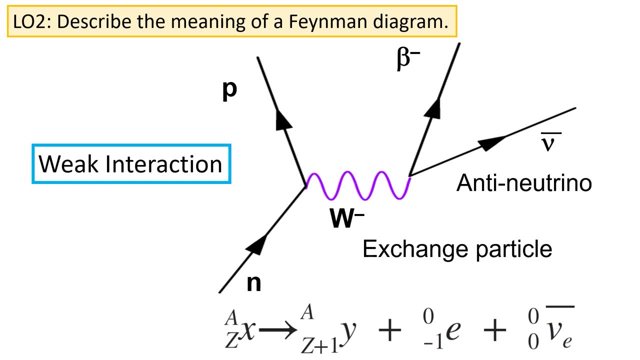 these are not included when we draw our Feynman diagrams. Let's look at an example of a process we already know about: beta decay. Beta decay is one example of a process which can be represented with a Feynman diagram. Here's the Feynman diagram for: 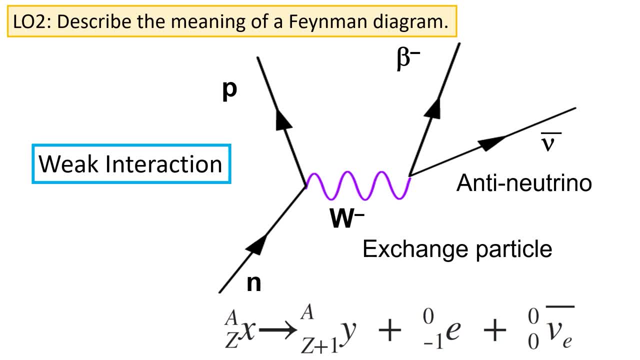 beta decay. We start with a neutron. This neutron decays and changes into a proton. As it changes into a proton, it also releases the exchange particle, in this case the W minus boson. This W minus boson then creates a beta minus particle, that is, an electron, and an extra particle called an antineutrino. 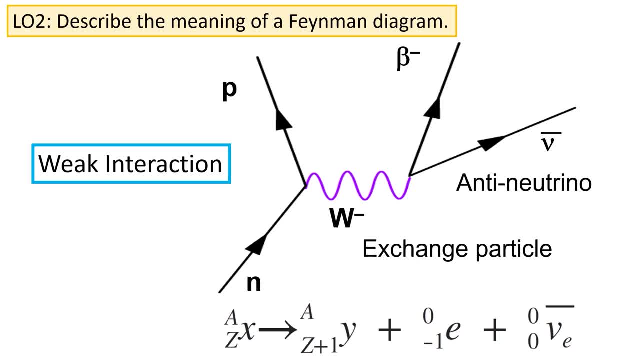 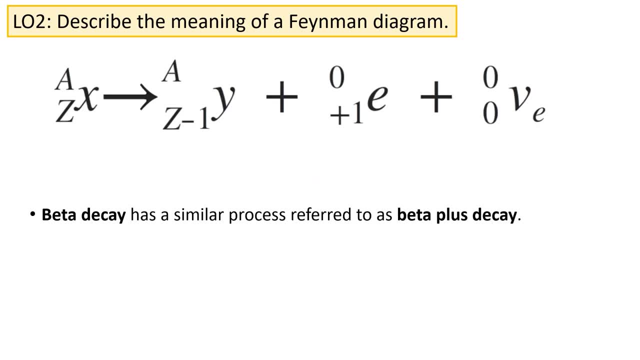 We've not met this antineutrino before, but we'll come back to it when we talk about conservation laws. There's another similar process to beta decay, called beta plus decay Instead, in beta plus decay, what happens is a proton changes into a neutron, releasing a positron and an neutrino. 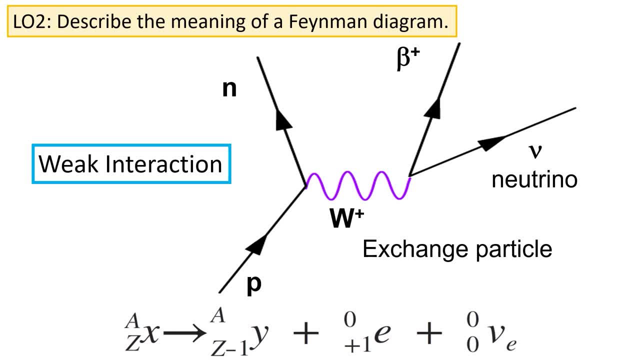 Here's the Feynman diagram for beta plus decay. Again we start in the bottom left, but this time with a proton. The proton decays into a neutron and a W plus boson. The W plus boson then itself decays into a beta plus decay. 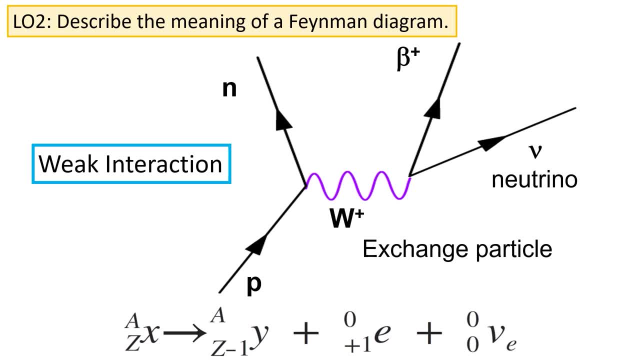 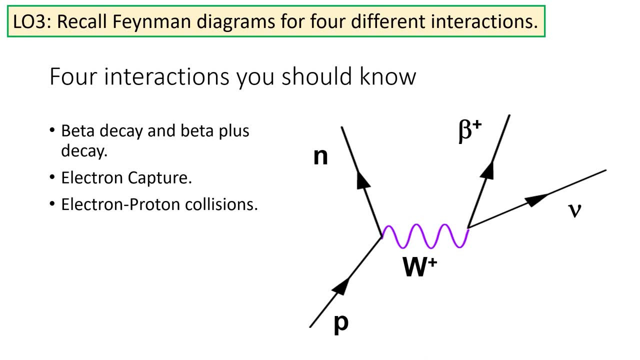 And these interactions simplify into an electron and an electron remains, so there's oneoul. You should know four different interactions like this for the exam. It's worth you memorizing these interactions so that you can state them quickly in the exam. These are beta plus and beta minus decay. 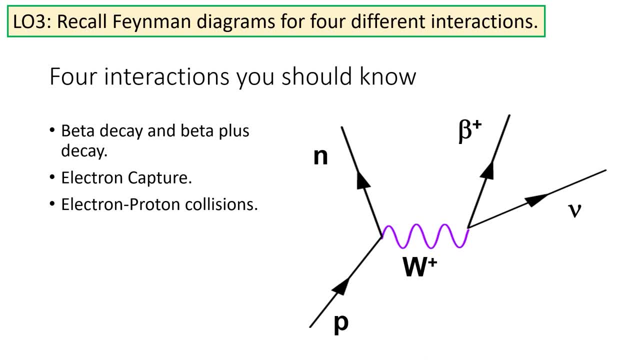 Electron capture and electron-proton collisions. Although that sounds like a lot, several of these diagrams are very, very similar to each other. capture With electron capture, we actually start with two particles, a proton and an electron. They interact through the weak interaction and we get a neutron and the emission of a neutrino. 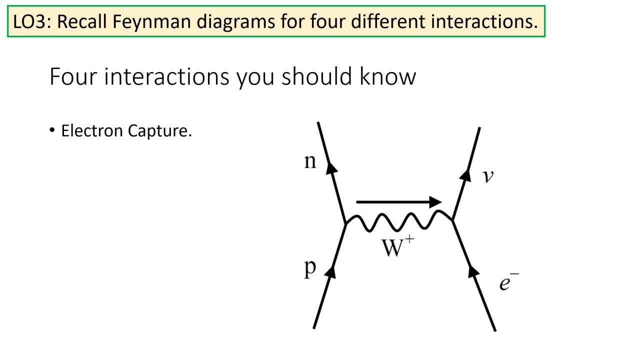 One important aspect to note is that the weak interaction with the W plus boson takes place from left to right. This is the opposite of what happens in electron-proton collisions. In the electron-proton collision we have something very similar. We start again with a proton and 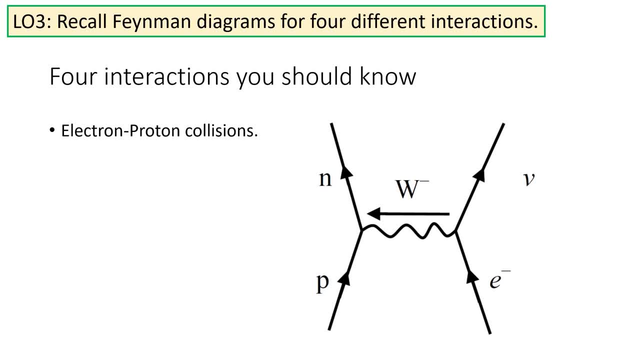 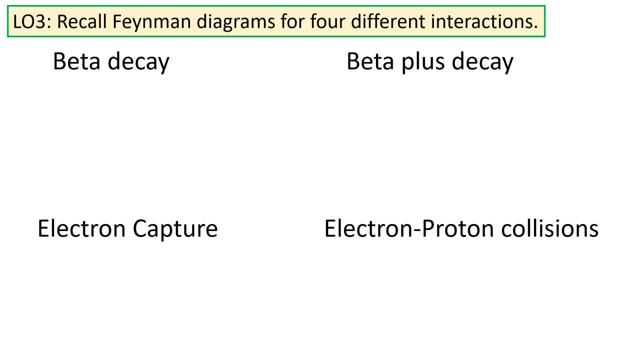 electron, but the interaction takes place right to left, and instead of the W plus boson we now have a W minus boson. These, taken together, are the four different Feynman diagrams that you should learn for the exam. Take some time now to pause the video and draw each of these Feynman diagrams in. 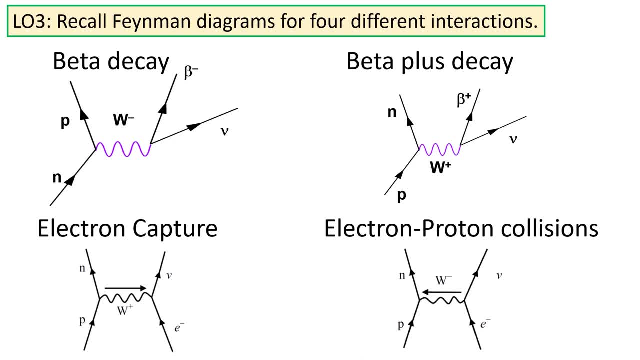 turn. Once you've done that, go back and see if you can redraw the Feynman diagram and diagrams without looking at them.